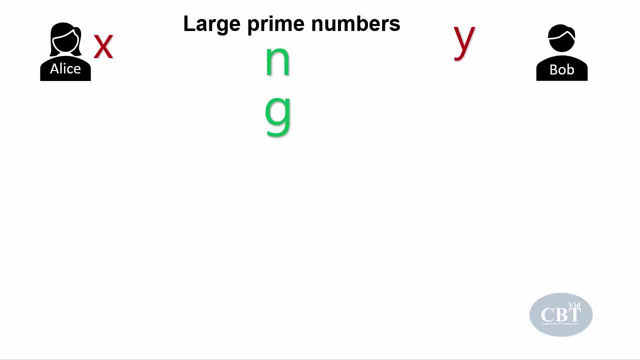 Then Alice and Bob both come up with two private numbers. In this case for Alex, we call that number X and Y for Bob. Now let's put some values to these X and G and Y, so that we understand the concept better And instead of using very large prime numbers. 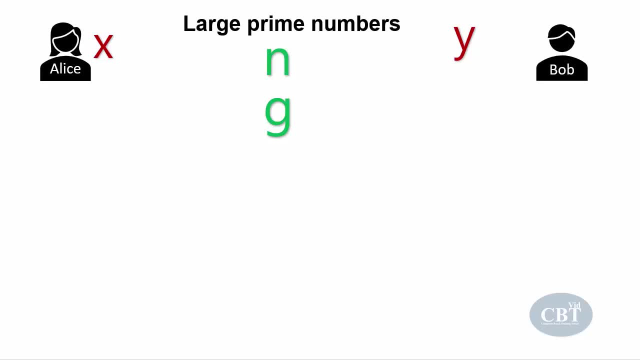 I'm going to use a smaller prime numbers because a calculation is easier and we're going to use that for the sake of understanding here. So let's say: for N we have 11 and for G we have seven. So these are two prime numbers and X is three and Y is five. 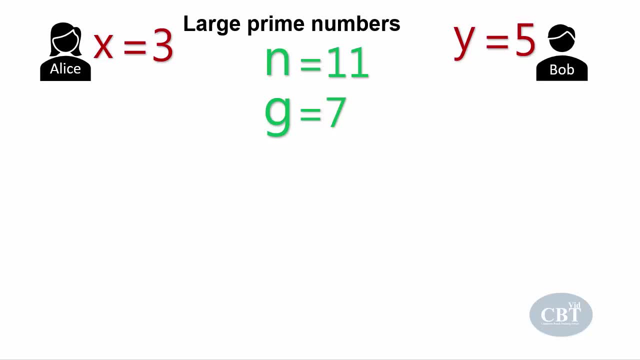 So Alice and Bob agree on these two numbers and they can exchange that over her X and Y phone or any unsecure channel, that doesn't matter. And even if someone knows about these numbers, that's okay. They cannot use these numbers to come up with a key. 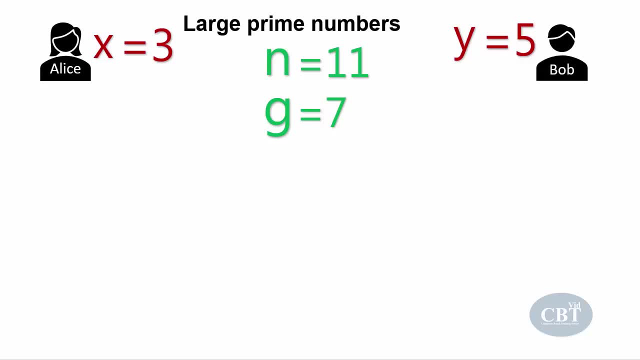 The most important thing is to keep X and Y private. Alice keeps X private to herself. She's not going to share that with anyone, including Bob. And Bob is going to keep Y to himself, and he's not going to share that with anyone, including Alice. 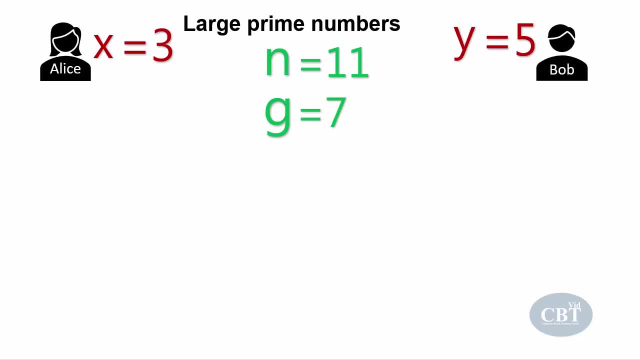 Now both of these two are going to use some formulas. Alice is going to calculate an A, and that A is G to the power of X modulo N. In our case, G is 7 to the power of X. X is 3 modulo 11.. 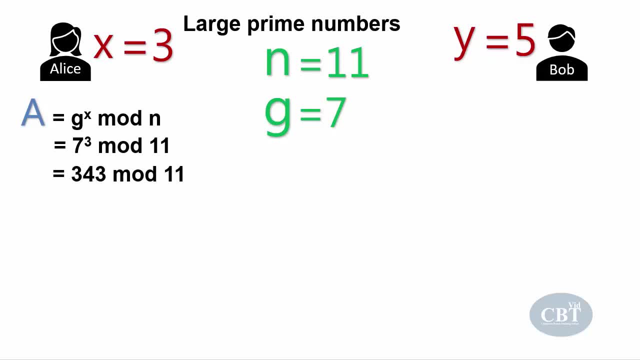 The result is going to be 343 modulo N. So that means we're looking for the remainder of division of 343 by E, 11. So the remainder is going to be 2.. Bob is going to do the same thing, So he's going to. 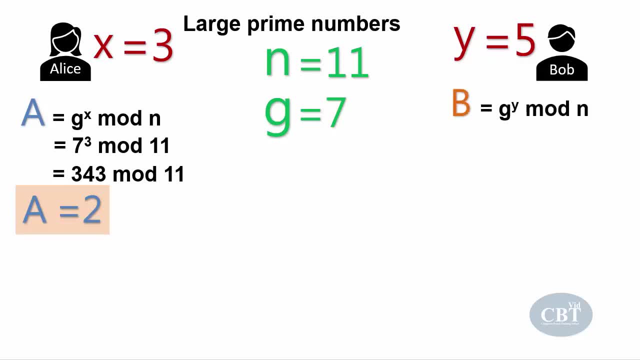 calculate a, B, and B for him is G to the power of Y, which is his private number, modulo N. So in this case we have G, which is 7 to the power of 5.. And 7 to the power of 5 is going to. 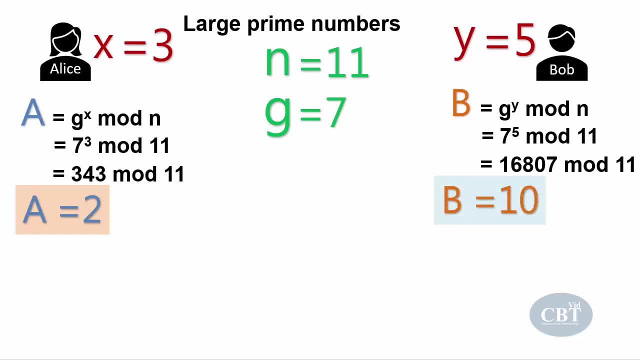 be 16,807 modulo 11.. So the result is going to be 10.. So the remainder of this division is going to be 10.. Then Bob is going to send this value to Alice and Alice is going to send her A to Bob. 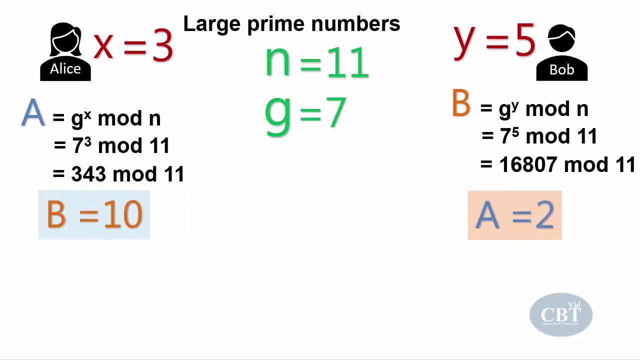 So they exchange these two numbers, Even if someone knows about this. it's okay because, as I said, they cannot use it. I'll show you shortly what I mean. Now, once Alice receives B, she's going to use another formula to calculate her key. So she says K is B to the power of X. 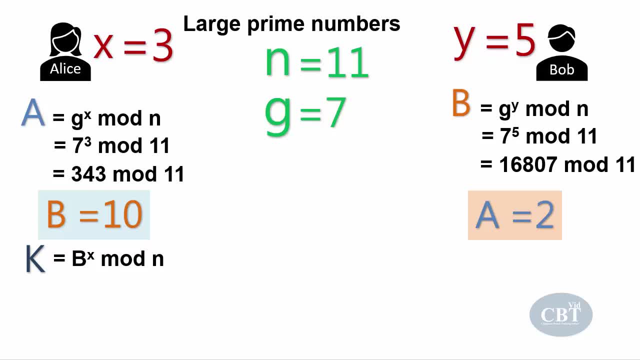 modulo N. B is the value that she received from Bob, And Bob is going to say: I'm going to calculate my key and my formula is A, which I received from Alice, to the power of Y, my private number, modulo N. So for Alice the value is going to be 10 to the power of 3.. That's 1,000 divided. 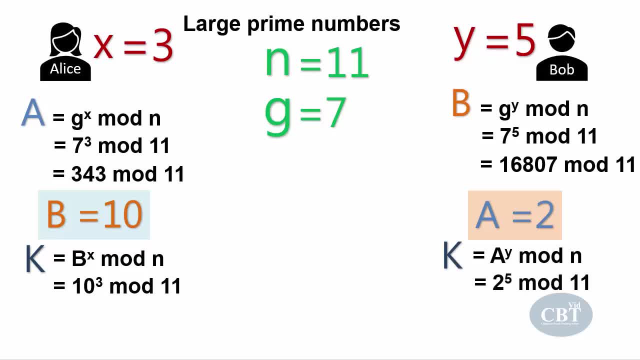 by 11.. And Bob is going to calculate 2 to the power of 5.. That is the value that he received from Alice modulo 11.. So 2 to the power of 5 is 32 divided by 11.. The remainder of these two equations is going to be 10.. So, as you can see, both of them. 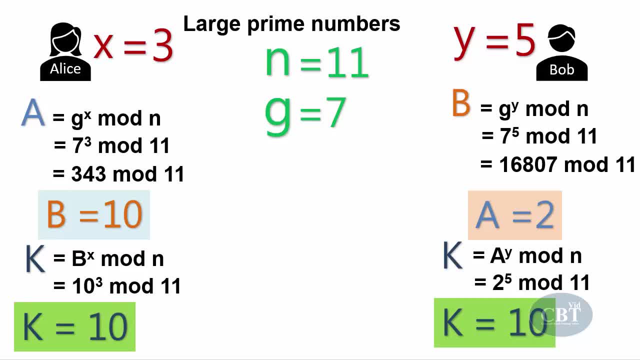 came up with a key which is similar, So that's how they exchanged the key. Now they have a key, Nobody knows about that key, And the key is exactly the same for both of them. Now you may ask: how is this possible? N and G- everybody knew about them, And later B and A also was exchanged. 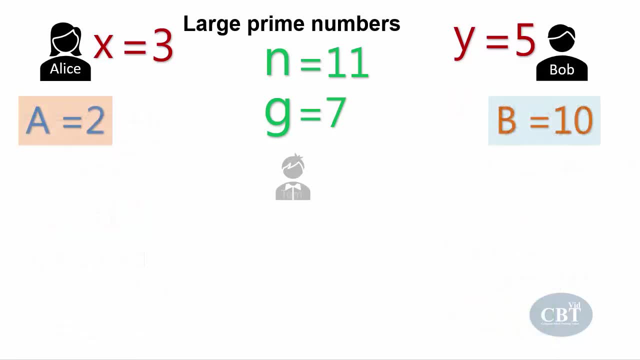 over on Secure Channel. So what if someone like Tom knows about these values? Can he use these values and calculate a key for himself? And that key is similar to Alice and Bob. Well, let's find out. Let's say Tom has a number that's a private number for himself, And that number is Z And 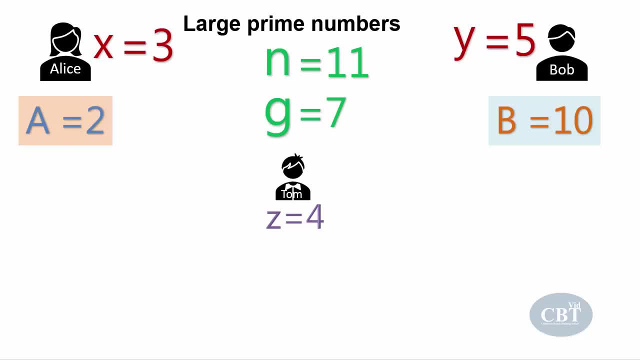 the value for Z is 4.. Now Tom's going to calculate a T And that T is G to the power of Z modulo N. So then Tom's going to say: okay, I know about G, So G, which is 7 to the power of 4, modulo 11,. 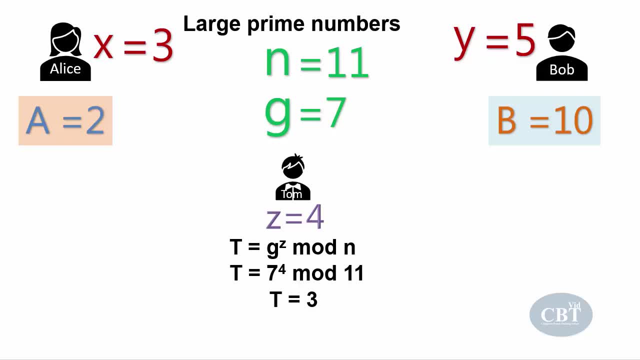 is going to give me 3.. Meaning 7 to the power of 4 divided by 11, the remainder is going to be 3.. Now, in the meantime, Bob and Alice have calculated their A and B, And now they exchange their A and B, And then they come up with their key, which is 10.. 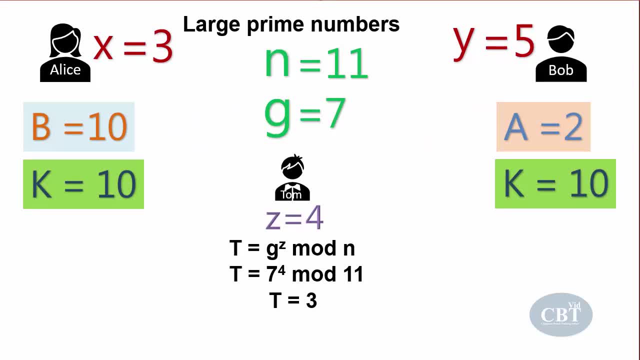 Now let's see if Tom can calculate the same values. So on Alice's side, Tom is going to use this formula: The B that Alice received from Bob to the power of Z, which is Tom's private number, modulo N, So that will be 10 to the power of 4, modulo 11.. And the result is 1, which is not equal to what. 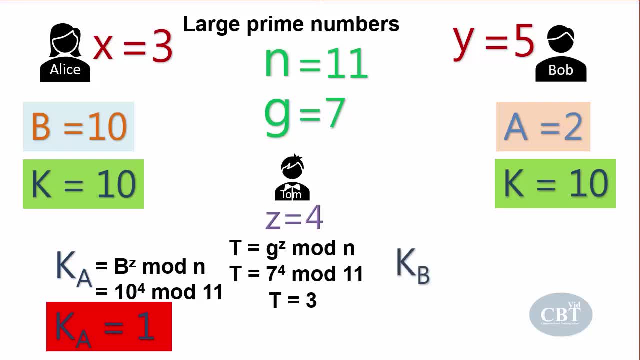 Alice calculated. Now on Bob's side, he's going to calculate another key, And that will be the A that Bob received from Alice to the power of Z modulo N, which is 2 to the power of 4, modulo 11.. 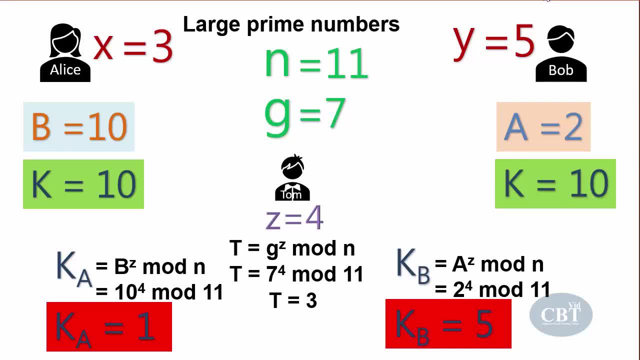 And the result is 5.. Now we can see. the two values that Tom calculated are not even close to what Alice and Bob have. He wasn't even able to calculate the same key values on both sides. So that's how Diffie-Hellman works and keeps your key secret. 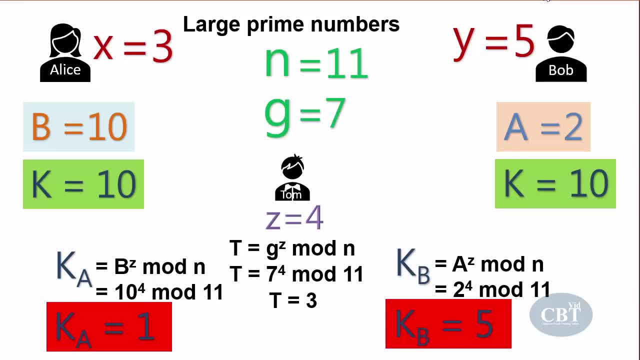 Now there is one way for Tom to get his hand on that key, And that's if Tom acts as man in the middle, And for that he needs to have two Zs, two private numbers- One for Alice's X and the other one for Bob's Y- And when Bob and Alice exchange those A and Bs, then he needs to stop. 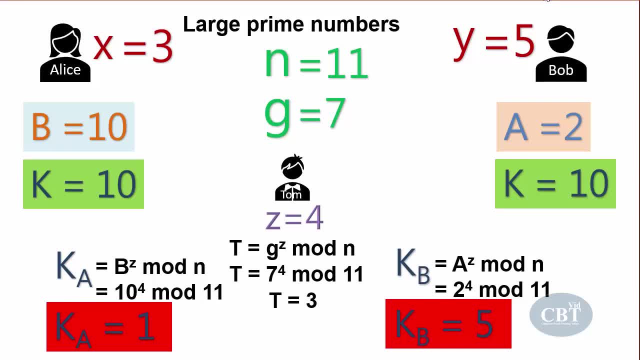 those and provides them with his calculation, So that Alice thinks the value that she gets is from Bob. but in fact it's not. So that's how Diffie-Hellman works. And that's how Diffie-Hellman works: It is from Tom, and Bob thinks the value that he got from Alice is from Alice. 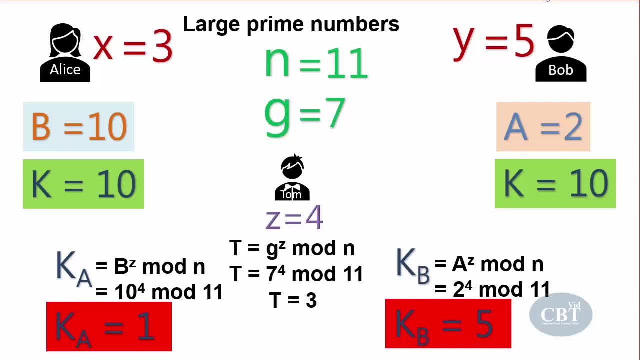 but in fact that's from Tom again. Now, when they come up with a key, then Alice's key is similar to what Tom has on the left side and Bob's key is similar to what Tom has on the right side. So Tom will have two keys: One is equal to Alice's key and the other